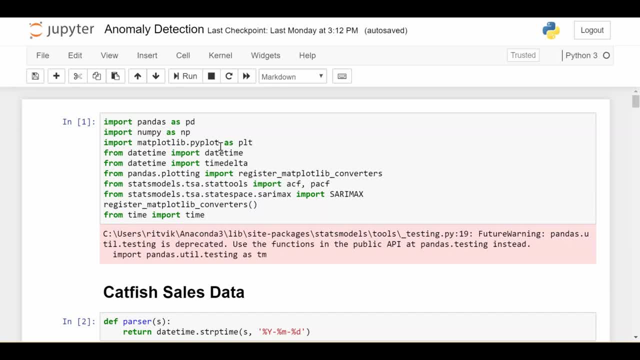 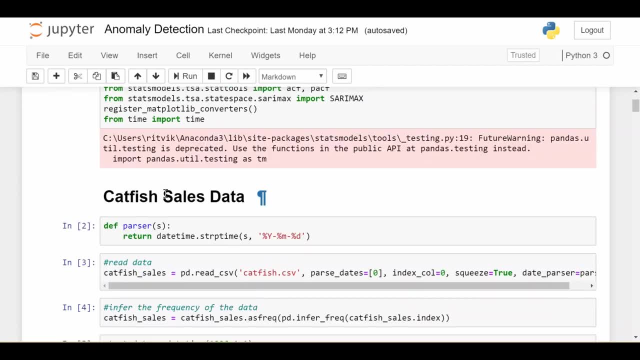 what that means visually and we'll see how to first detect it and then how to account for it, so that we're not getting really bad results in our predictions. We'll be looking at the same catfish sales data we looked at in some previous videos. This data will be linked in the description. 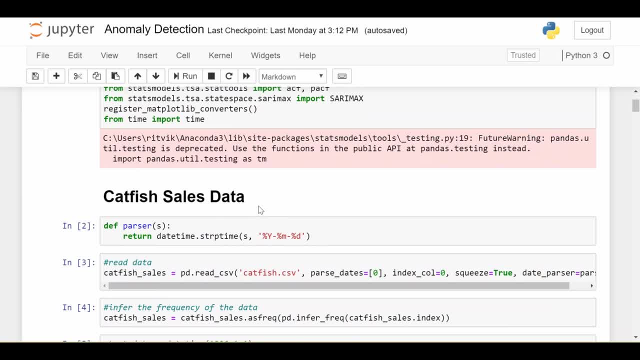 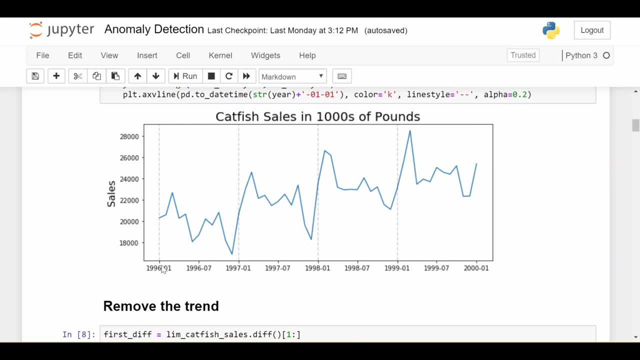 and this notebook will also be linked in the description So I won't go through all the stuff we went over before. This is how the data looks. We've taken a snapshot of the data to analyze from 1996 January until 2000 January. So we have these four years of data. We see there's a clear 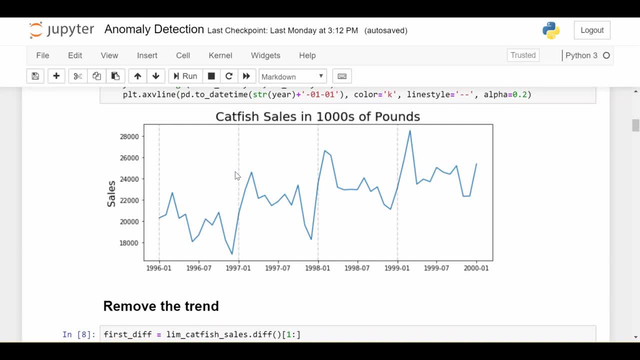 seasonal pattern between these gray dashed lines which separate years, And we should be able to exploit that seasonality. And we're going to build a SARIMA model which is a seasonal autoregressive integrated moving average in order to predict the last seasonality. And we're going to build a SARIMA model which is a seasonal autoregressive. 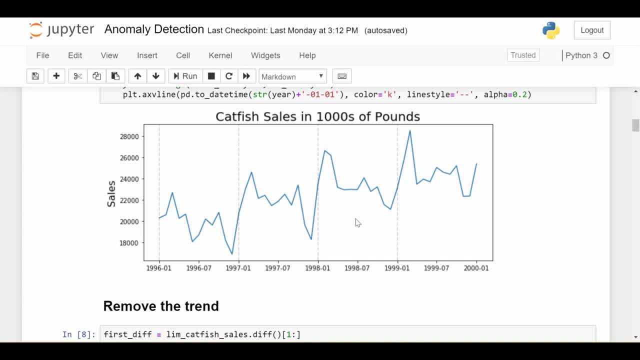 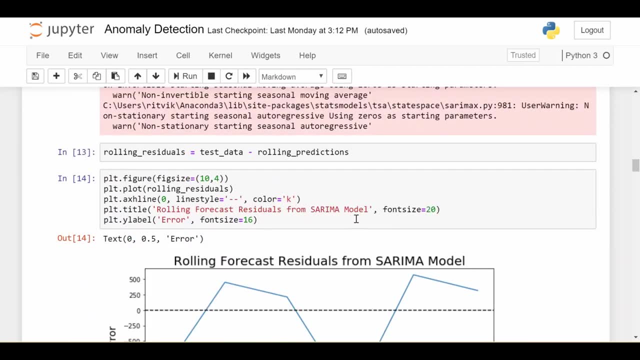 integrated moving average in order to predict the last six months, given the first three and a half years. So again, the code that's coming up here is basically just the prediction, which is all content in other videos, But suffice to say, when we use a rolling forecast origin to predict our 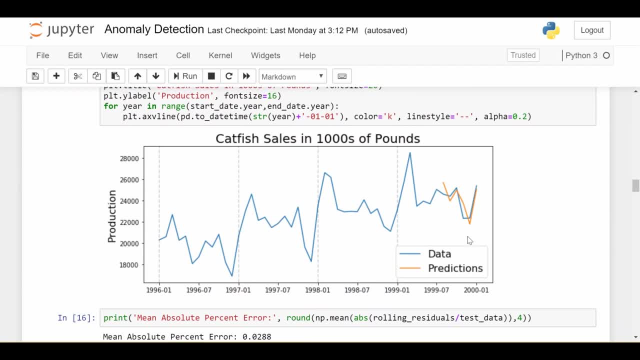 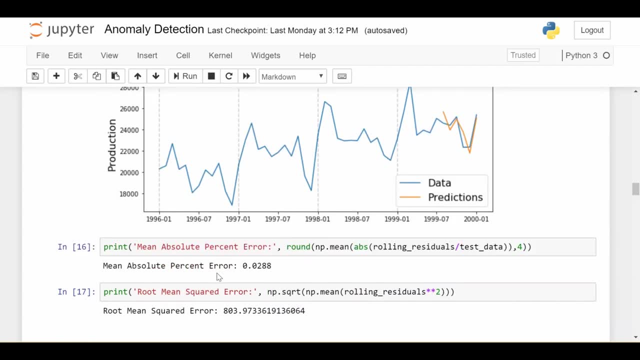 six months. this is what our prediction looks like. So the orange line you see here is predicted and the blue line is the data. So we see it's not bad, pretty good actually. We see the average percent error is 3% and we see that the root mean squared error is just around 800.. So I'd say this: 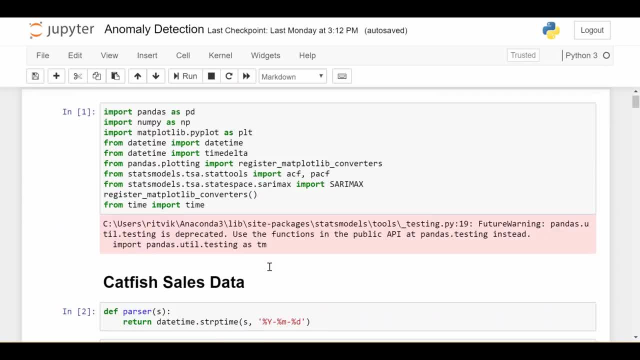 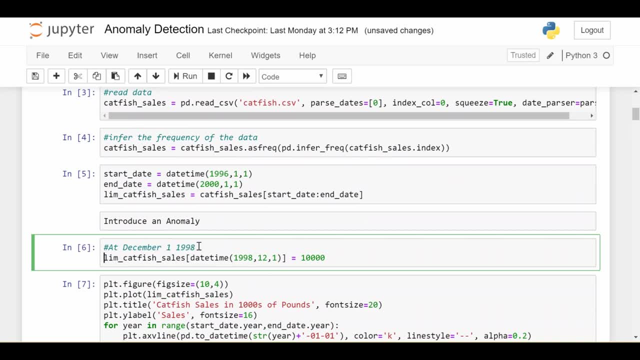 is a success. Now here's where the trouble is going to start coming in. I'm going to artificially introduce an anomaly, So I'm going to set December 1st 1998, I'm going to set that data point to a value that we would not expect. So I do that First thing. we'll look at how the data looks. So 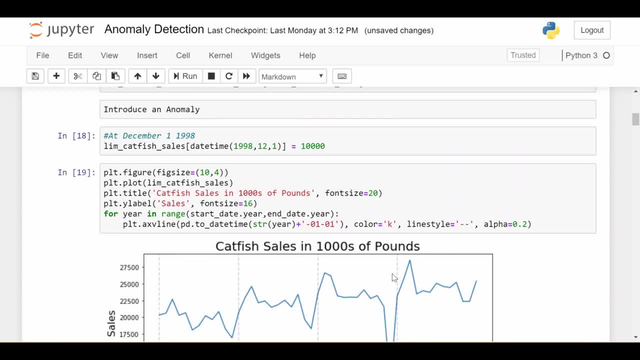 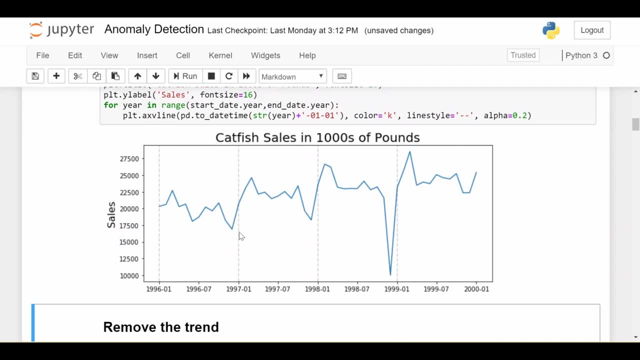 very obvious where the anomaly is. So right here at December 1st 98. And we see that we would expect this value to be maybe around the December value here. the December value here maybe a little bit lower, But we would not expect it to be this low And as weird as this anomaly looks. 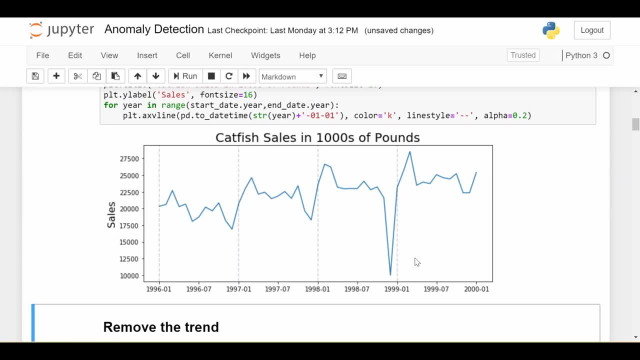 it's not something that's impossible in the real world As much as you expect something to be seasonal at all times. sometimes a big event happens in the world that just breaks that seasonal pattern. In fact, we're in the middle of one of those big events right now with the 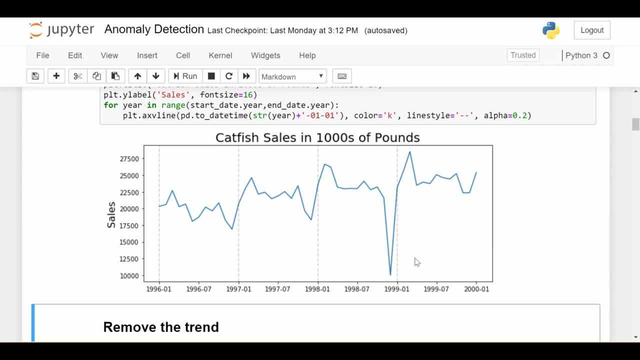 coronavirus crisis. I would imagine many, many time series that people are looking at have been disrupted by the current crisis and crises that have come before and crises that have come after. So it's up to us, as the statistician or the economists, to figure out how to first A detect that there's an anomaly here and 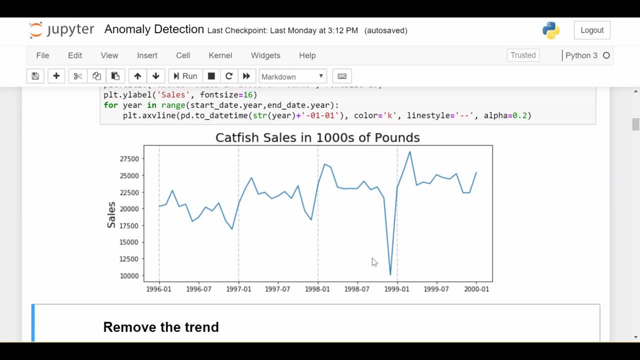 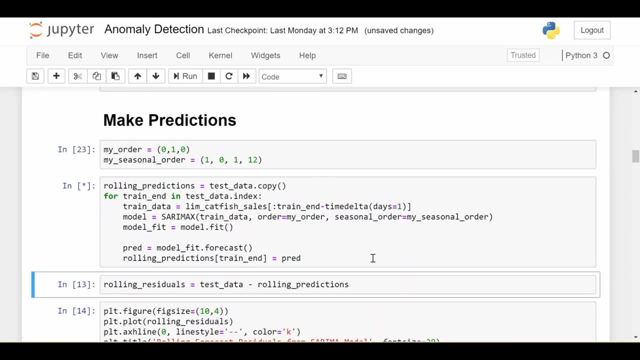 secondarily, how to correct for it so our predictions aren't screwed up. The first thing I want to show, though, is what if we fail to detect the anomaly? What if I just run the same code below and assume that everything's going to be fine? Then we see our predictions look like. 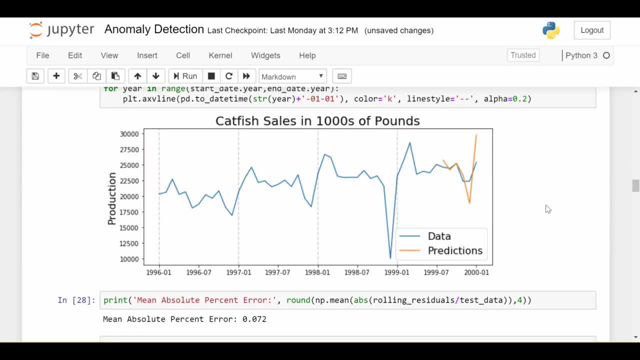 this, So they've been highly skewed. We see, the first couple months are actually okay, But as soon as we get to the December time point here, it's been highly underpredicted. And that makes sense, because it's using the same December data from this point, this point and this point. 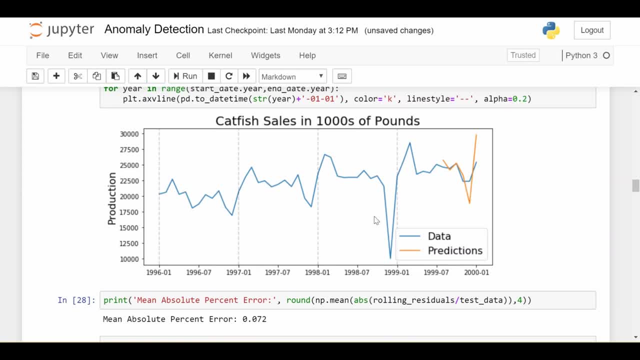 So it thinks that it should predict something really really low, But in reality this was just an anomaly in this year And because of predicting that really low, we then overcorrect and predict the next month really high. So this is going to be propagating the problem forward, And that's. 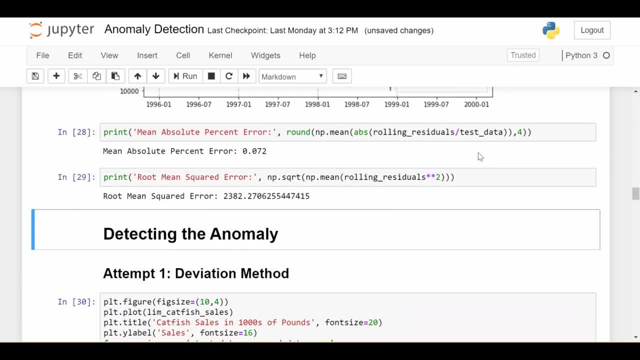 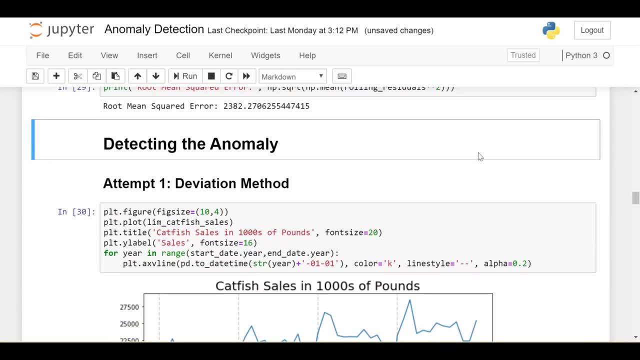 not something we want. So first we need to detect the anomaly. How are we going to figure out that there is an anomaly? Because before we remove it, we need to know it's there. We'll look at two attempts, one of which I think is strong. We're going to look at the first one, which is the. 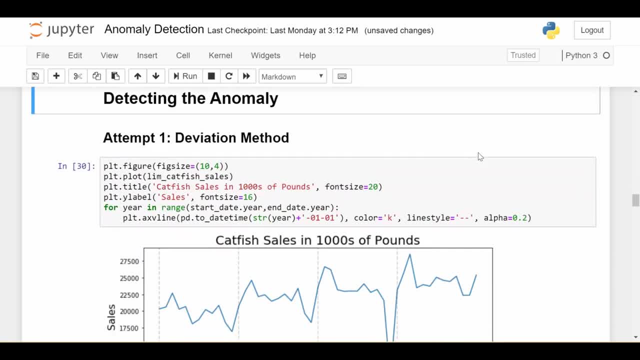 first one. So we're going to look at the first one, which is the first one, which is the first one than the other. The first attempt, which is kind of naive, is to use the deviation method. I can explain this pretty easily. So here's the time series. again, Let's say that we start looking. 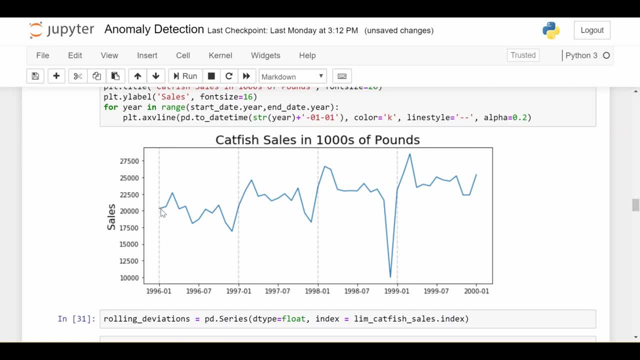 at the beginning of the data and then we basically just have a ever-expanding window. So first we look at just the first data point, then we look at the first two, then the first three and we just have this window expanding And for each window size we calculate the standard. 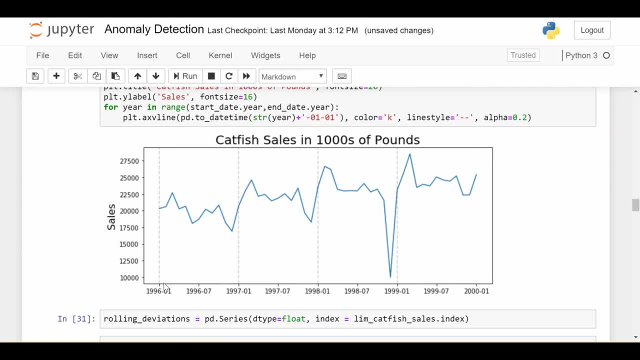 deviation of all the numbers in that window. So let's say our window is currently this whole first year, We would calculate the standard deviation of these 12 data points. If our window is now the first two years, we would calculate the standard deviation of these first 24 data points. 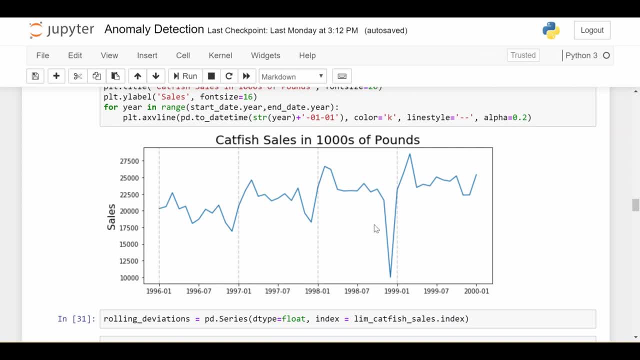 and so on. And the reason we're doing this is because, when we get to the anomaly, our standard deviation is going to go way up because we found a value that's out of the average, out of the norm. So, basically, if we plot the standard deviation over time, we should be able to use this as a 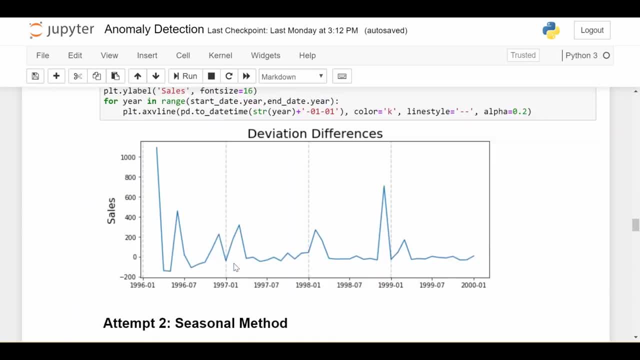 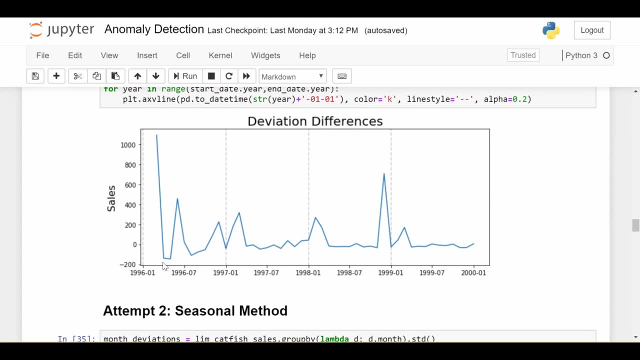 sort of anomaly detection method. So that's what I've done down here. This is the standard deviation over time. Now, one thing to note is that we kind of have to ignore the first couple, because when you take the standard deviation of just two or three numbers, the variation is going to be. 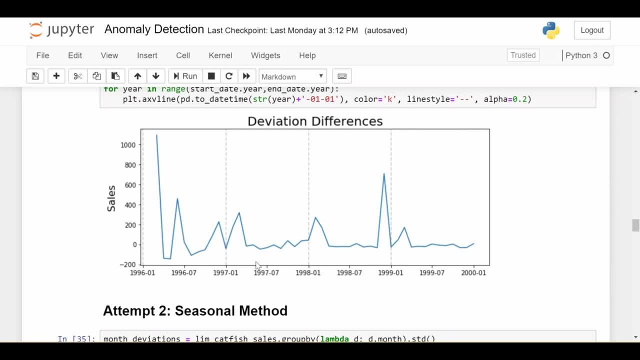 pretty high just because there's not too many numbers. So, although the highest point on our graph is actually the first one, it's not really high because it's an anomaly. it's high because there's not a lot of data. So that's one of the drawbacks of this method is it's difficult to 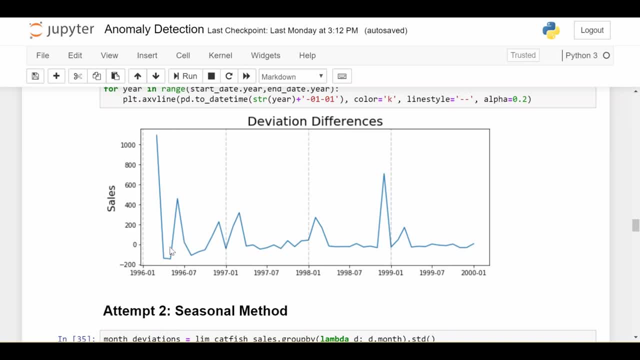 use it if the anomaly occurs very early on. But if we just kind of burn out the first couple data points- let's say we just start looking at this gray bar in the second year- then we see that the highest point clearly is December 1st 1998, which is exactly where the anomaly is, And again the 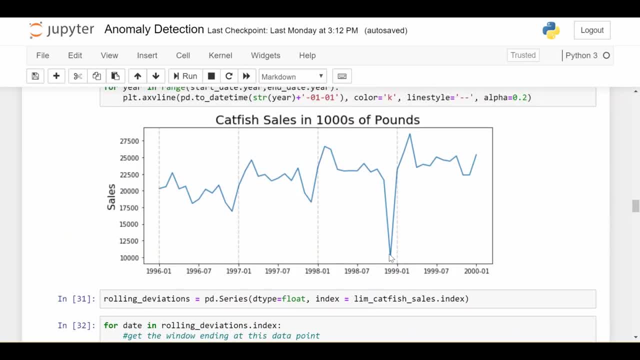 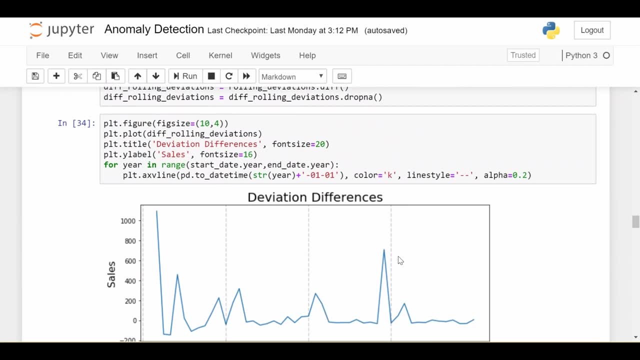 intuition is that when we reach that anomaly, the standard deviation of the series goes way up because we found a value that is very out of the ordinary. Now, as intuitive as this method is, obviously there's drawbacks, and the one drawback is obviously that the first couple data points 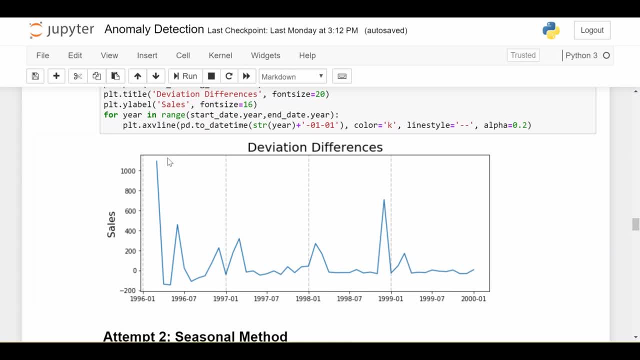 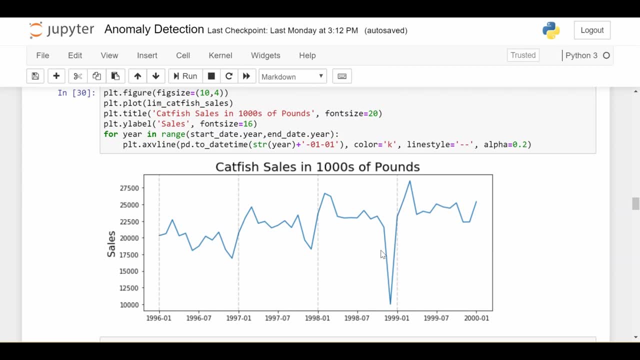 can't really be used as anomalies. So we're going to explore that with this method. and there's other drawbacks too, because anomalies aren't necessarily just very extreme values. they can be sometimes just unexpected values for other reasons. So let's look at a slightly more robust method. Let's look at the seasonal method. So this 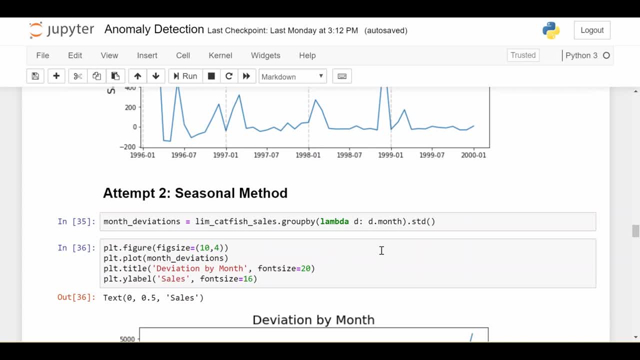 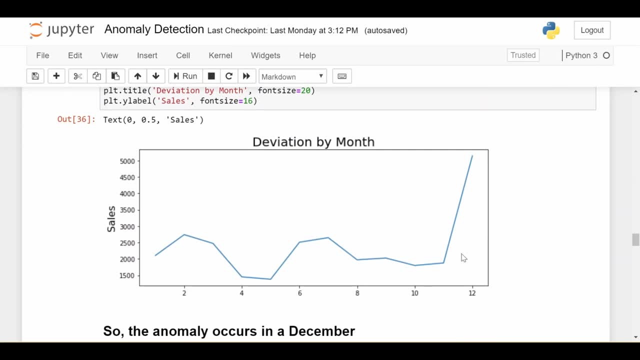 is exploiting the idea that we know that there is seasonality in our data, so we're going to use that fact to help us out, And this is also somewhat intuitive to explain. So the chart I'm about to show you, this chart basically shows me what's the standard deviation if I look at only data points. 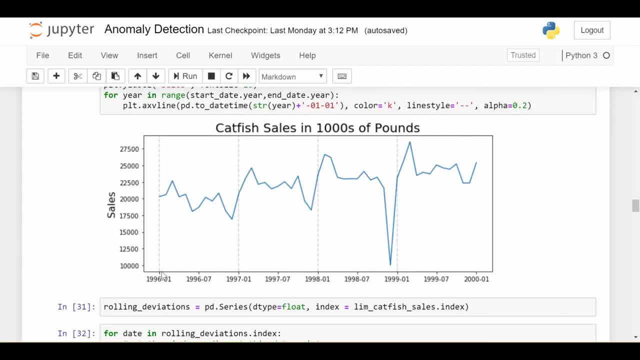 in the chart. So if I come back up to our main plot here, let's say I look at just January, so I'm looking at this data point, this data point, this data point and this data point. So I'm looking at the four January. 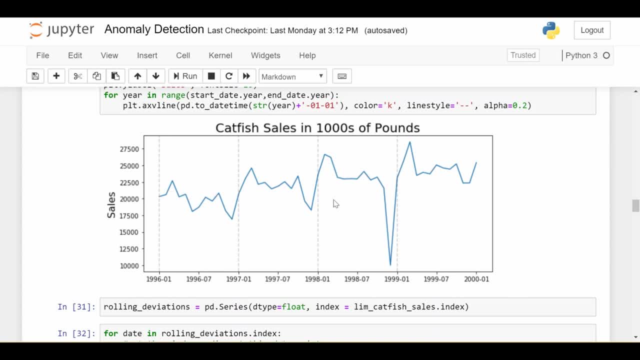 observations I have and I'm calculating the standard deviation between them. I would expect this deviation to be rather low Because, since I am assuming there's a seasonal pattern, I'm assuming that Januaries are pretty correlated with each other, Februaries are pretty correlated with each other, and every month. 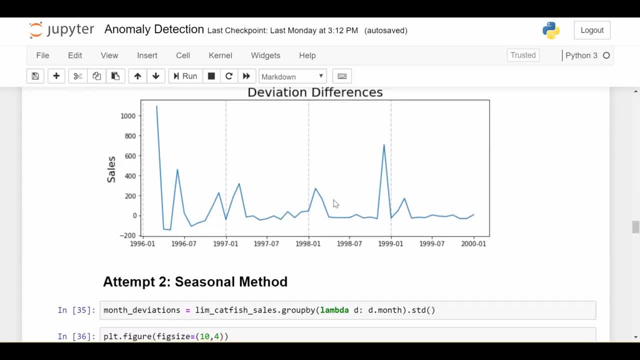 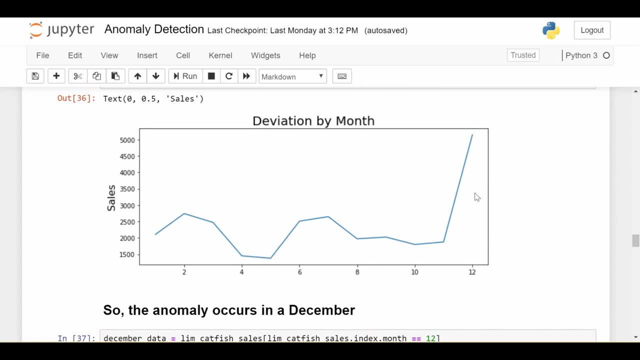 is somewhat similar to the same month in different years. So if I plot that deviation by month, we see most of the months have somewhat of a usual deviation. but when we get to December the deviation jumps way up. And that makes sense because we're taking 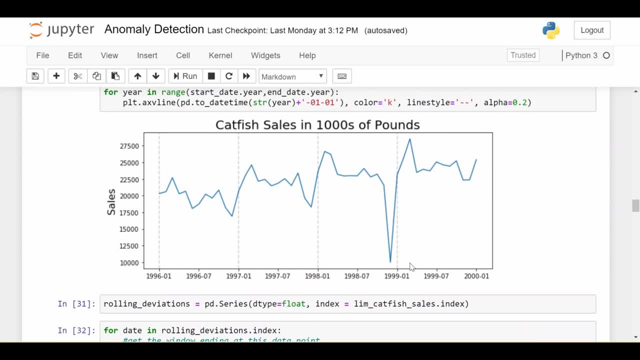 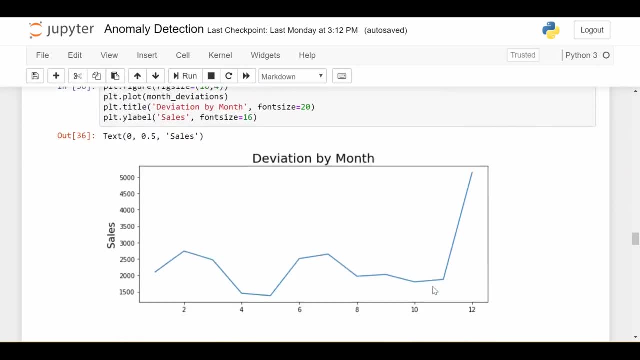 the standard deviation of this December, this December, this December and this December. So we see that there's a lot of variability due to the anomaly. So, based on this plot, we know that if we're looking for an anomaly, we should look in. 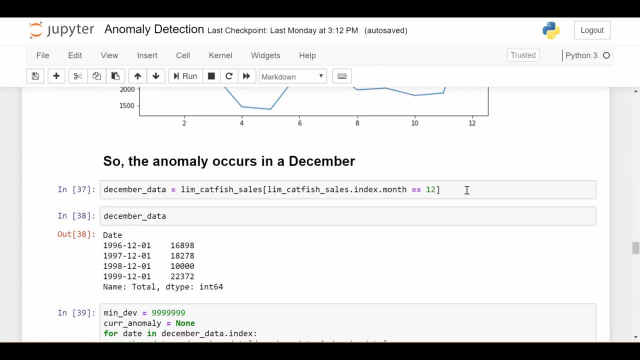 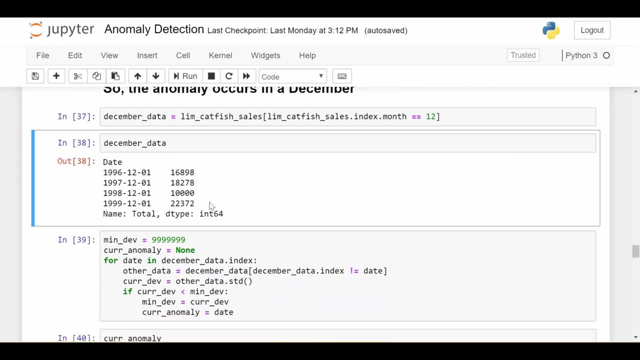 a December. So the stage two of this method is that we need to figure out which December the anomaly occurs in, and basically what I've done here is subset the data to look at just the four Decembers. Obviously, the anomaly is this very, very low number over here, but to solve that in terms of code it's also 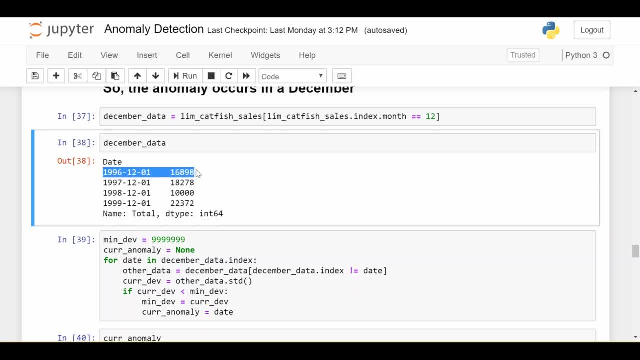 very simple. I basically just eliminate one observation each time and then calculate the standard deviation of the remaining ones. And if I were to look at the step where I've eliminated this observation and calculate the standard deviation of the other three, which are like the usual Decembers, then I would 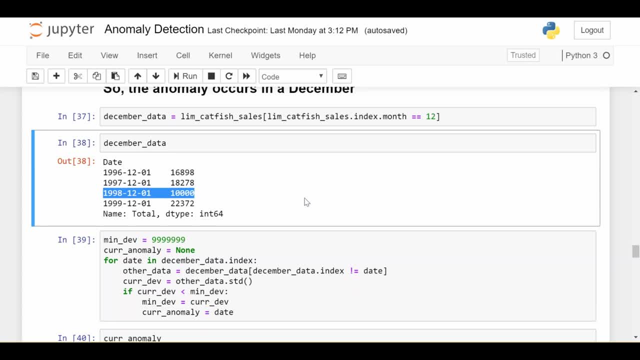 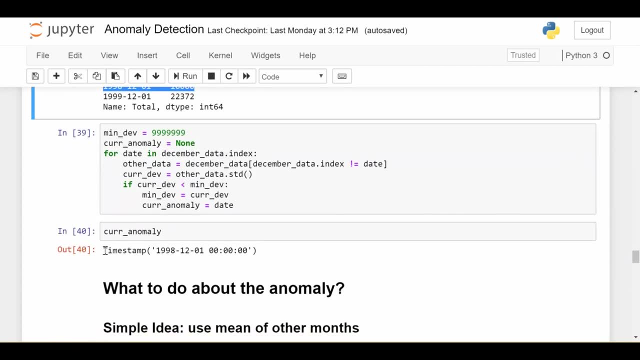 get a very small standard deviation. So I figure out in which case I get the smallest standard deviation and the number that I've left out will be the anomaly, And in that way we're able to identify that the anomaly occurs at December 1st 1998.. So this is our more robust anomaly. 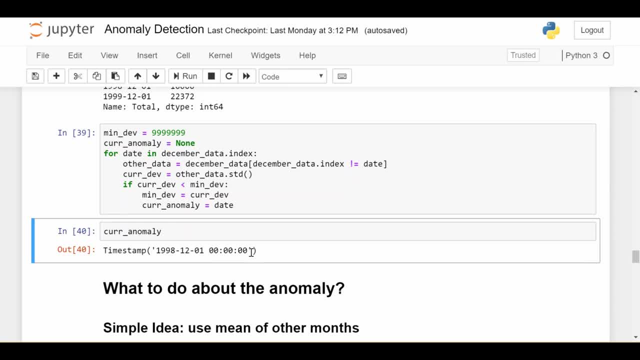 detection method. Now, before we go on to what to do about the anomaly, I should note that there are many, many more, even more robust anomaly detection methods, but I wanted to just expose you to a couple of options that you have And, if you are interested, please let me know in the comments and I'll make more videos. 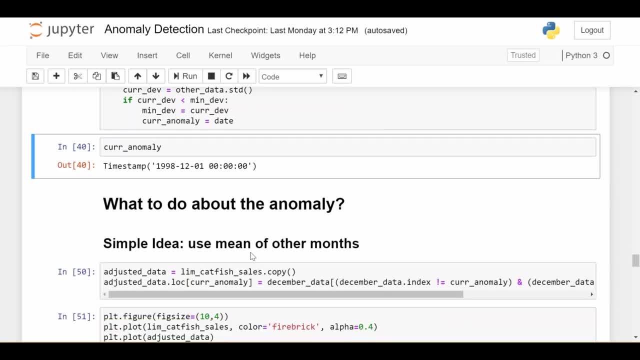 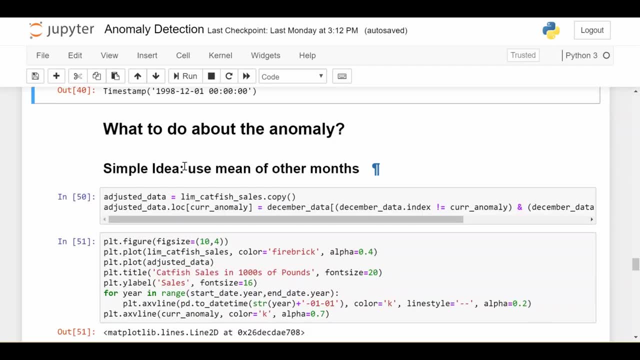 on robust anomaly detections. But to close out this video, let's see what to do about the anomaly. At this point we figured out that the anomaly is in December 1st 1998.. Here's the simple idea we'll look at to close this video out. 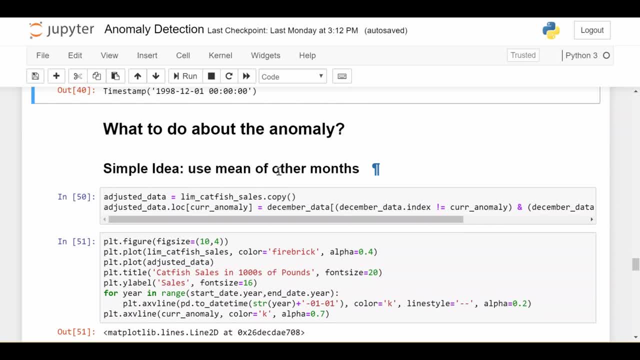 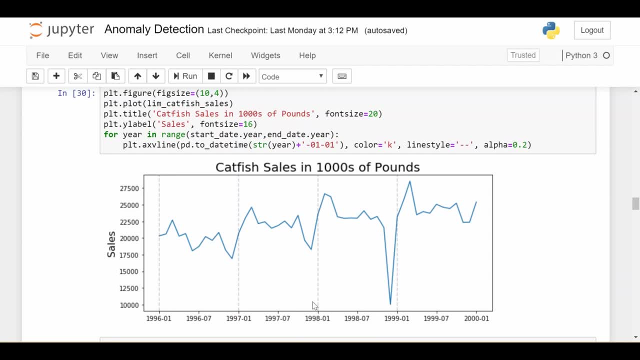 We're just going to use the mean of the other Decembers. So, looking again at the graph, I figured out the anomaly is here, so I'm going to use the average of the other Decembers. I'm looking at this one and this one. I'm not looking at this.